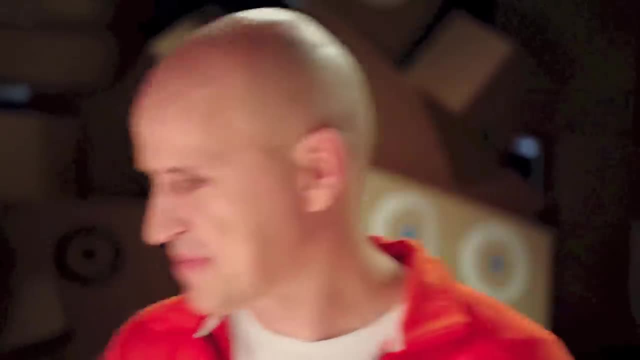 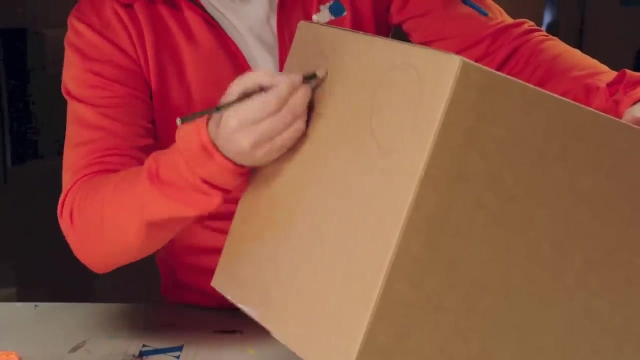 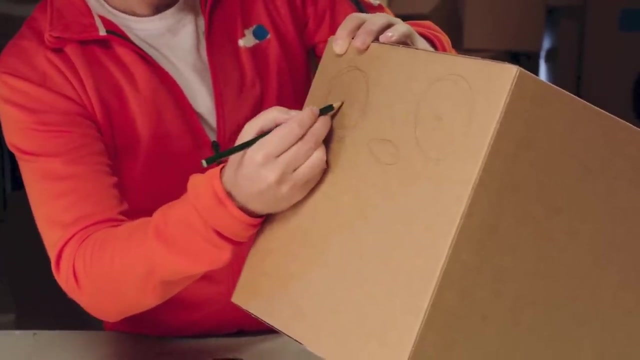 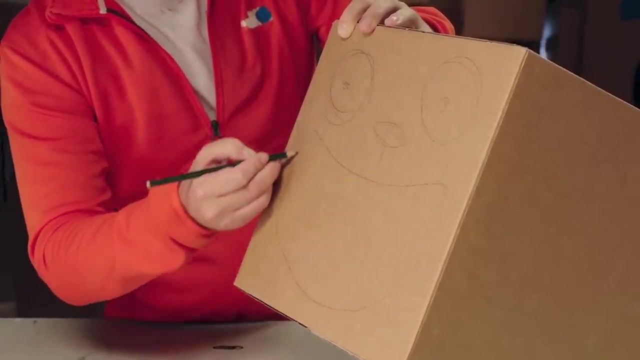 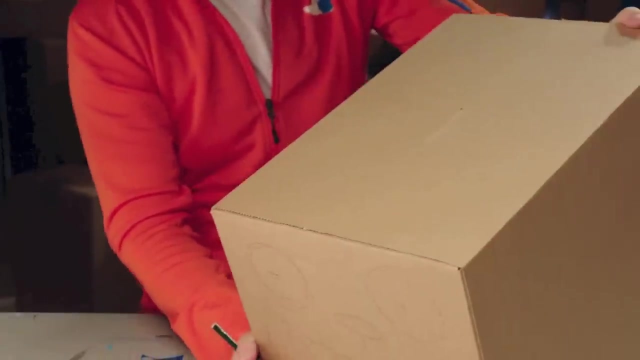 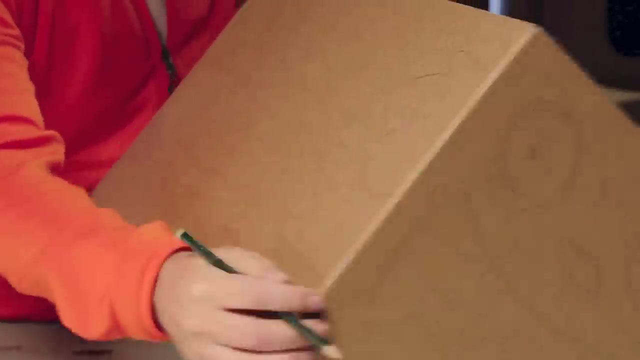 the drawing onto the box, one side at a time. Let's start by drawing a face on the front of the box: Eyes, Nose, Pupils And a big open mouth. Two big teeth And a big mouth, Some ears on the top And on the sides. draw some thick hair. Now let's draw a big window. 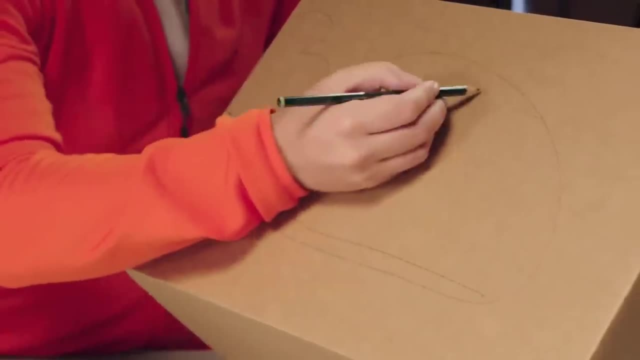 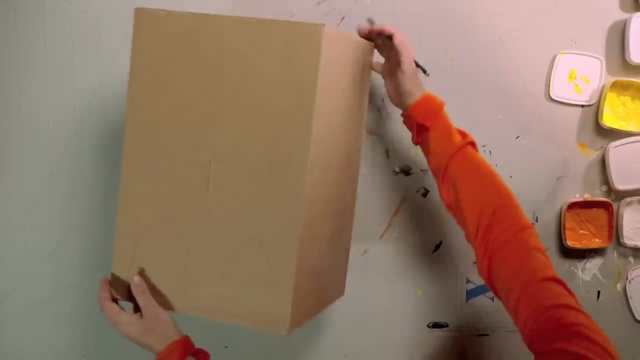 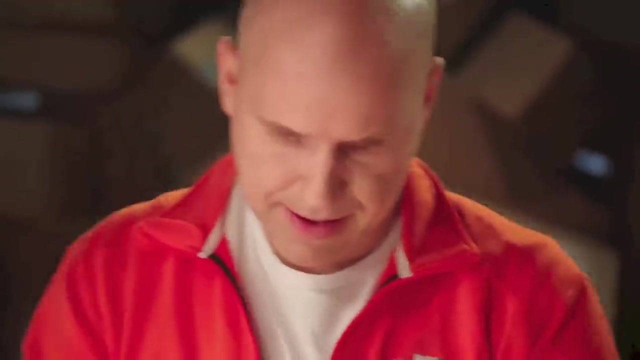 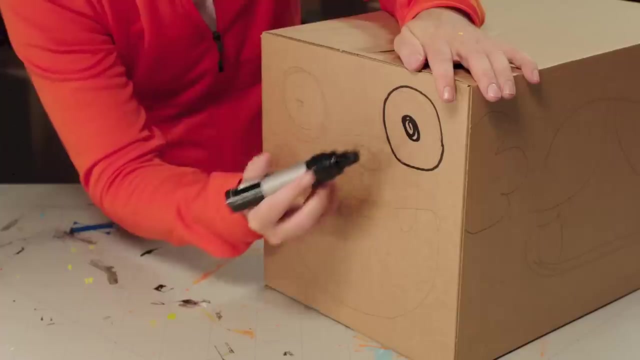 along one side With curtains, of course. On the back of the box, draw a tail hanging slightly to the right. Now get a marker pen and go over all the lines. It's good to draw with a pencil to start with. Then it doesn't matter if you get something wrong, Only when you're completely. 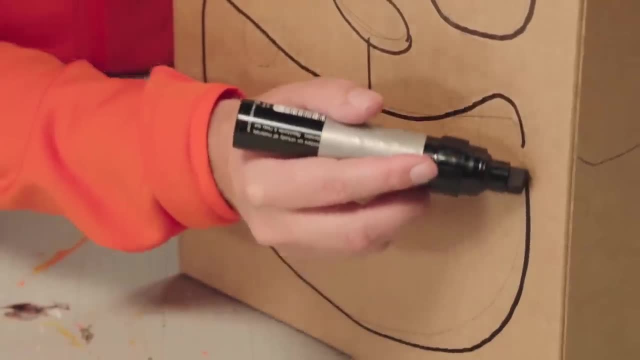 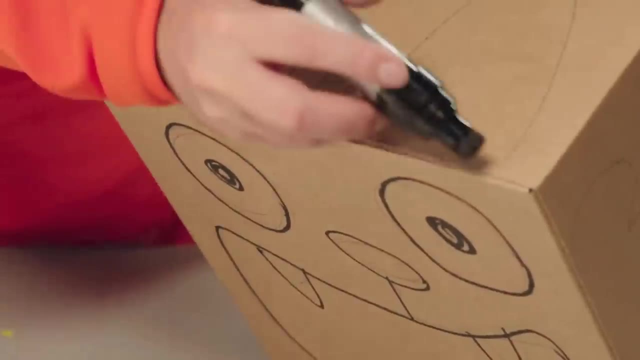 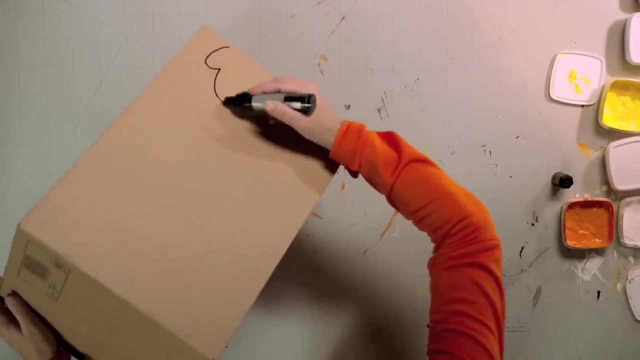 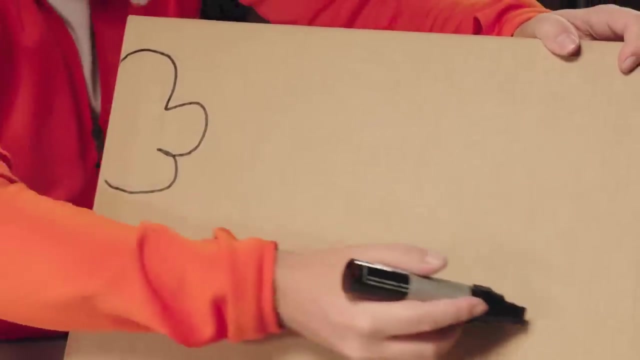 happy with your pencil drawing. use your marker pen to make the lines thick and strong. Try to find a waterproof marker so the lines don't dissolve when painting the box, Because building a literal painting doesn't mean the words areары. the lines don't translate. 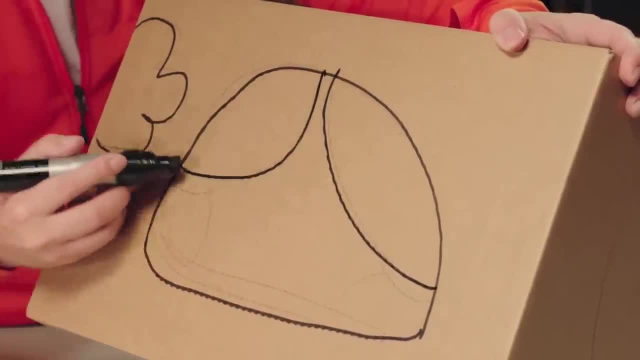 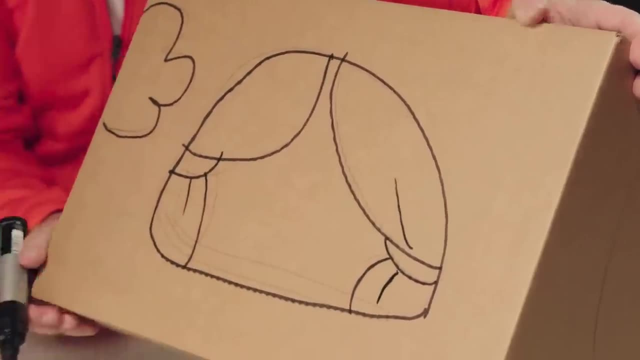 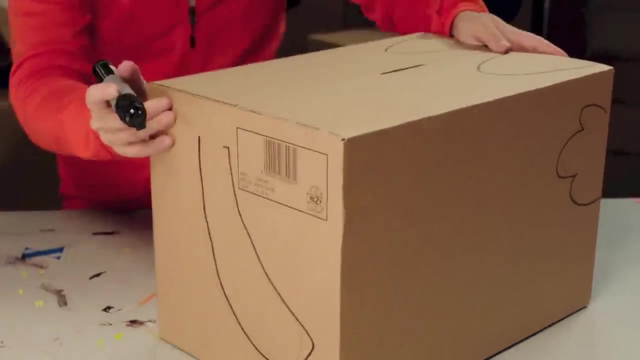 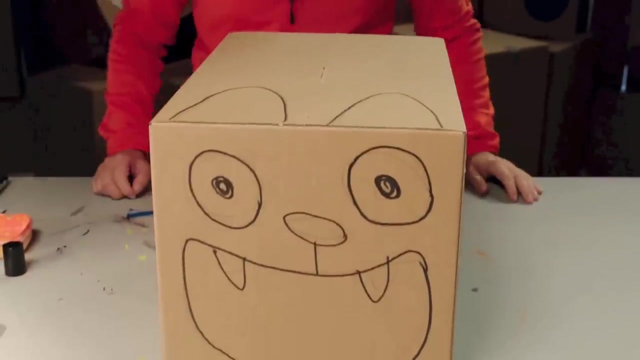 out dunno. So we'll do the affectionately dark brown together on the cover. Now, soft-tape, paper ぎ. What? Doesn't it have an 초� comeback? No, That's the drawing done, Nice and easy Paint. 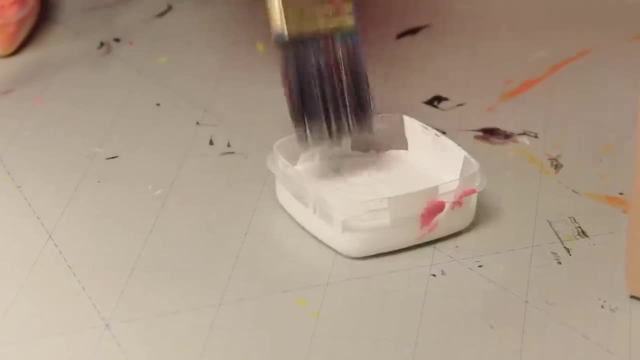 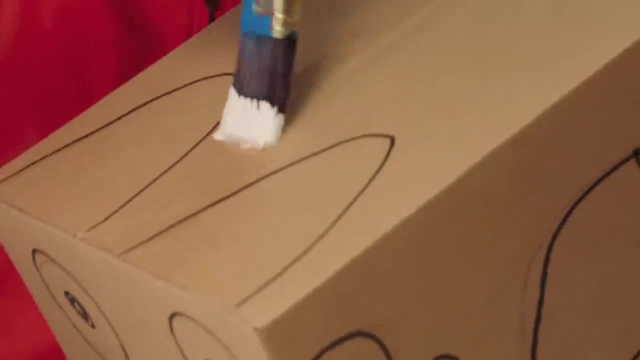 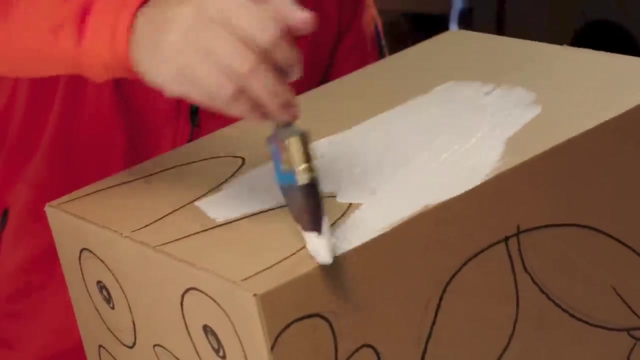 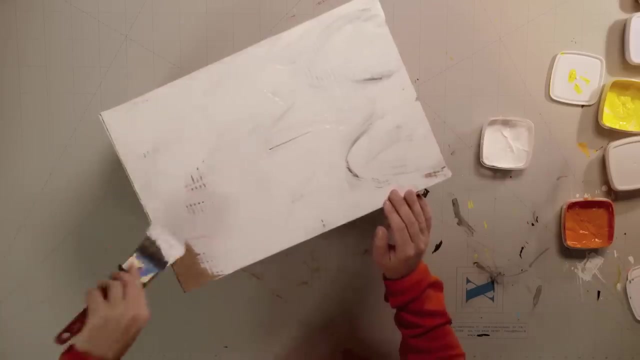 And now we can paint it up in bright colours. Go for it with a big, thick paintbrush and white paint so you can cover the whole box as quickly as possible. Don't worry about painting over the marker pen lines. These will show through the paint when it's dry and we can touch them up again later. 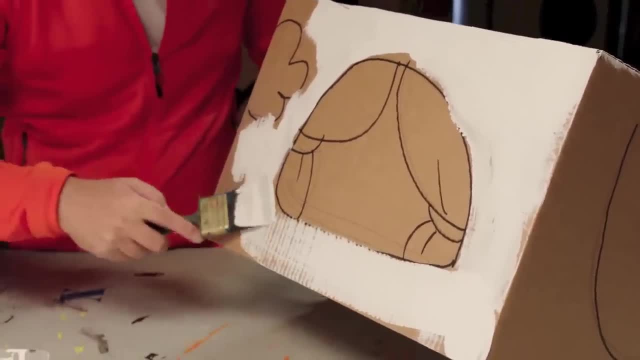 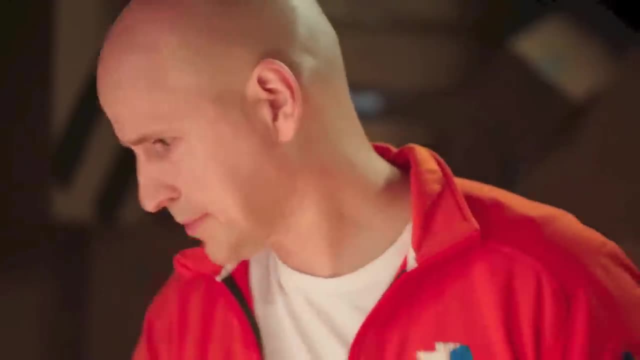 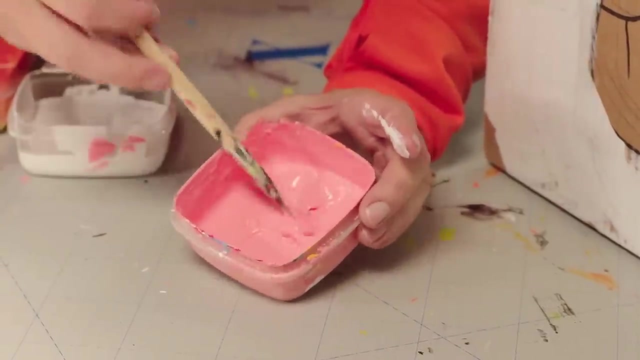 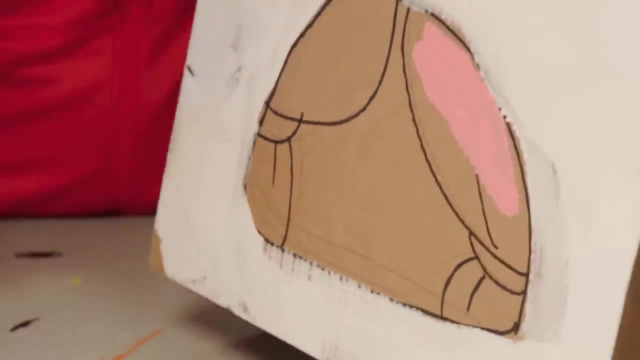 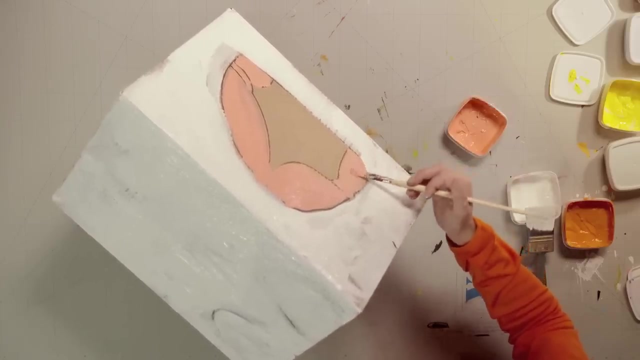 The white is what we call a primer, so the other colours painted on top look even better. Now for some pink. Use this on the curtains to make a holy and cosy feeling for the cat house. Let's get rid of that box and replace it with this one which has dried. 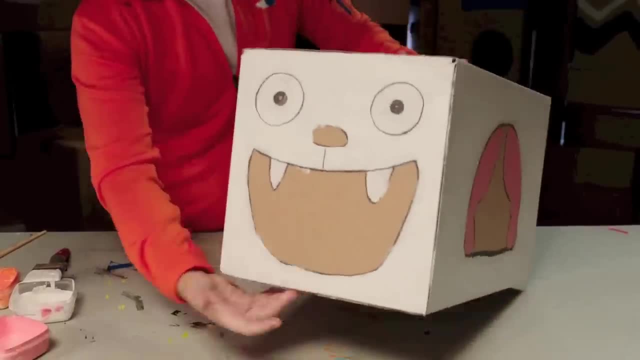 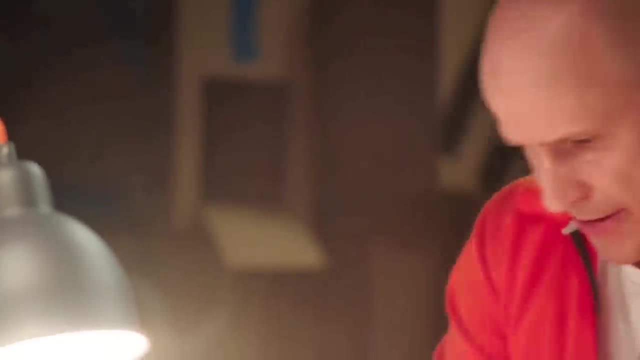 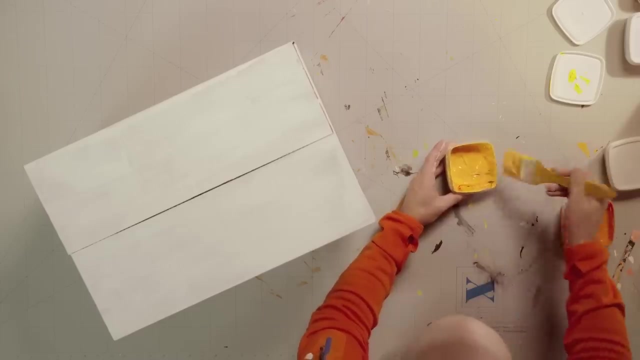 It looks almost like a ghost cat white all over. So let's fix that with some paint, More paint. I'm mixing a dash of red into this yellow paint to get a sharp and strong orange colour. Paint that on the sides, but be sure to leave a stripe of white along the bottom. 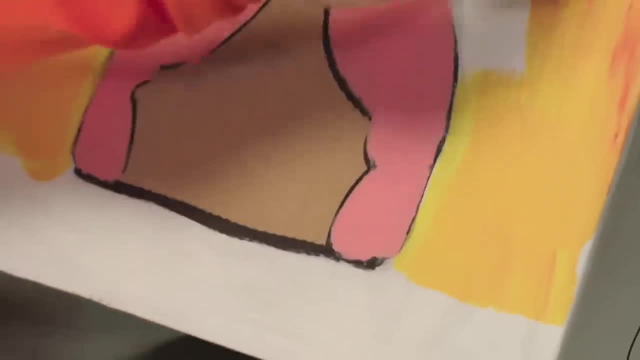 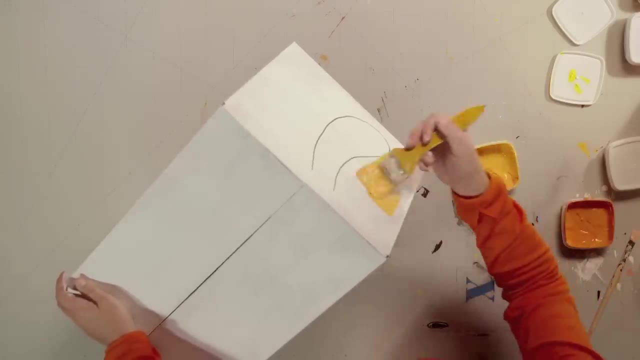 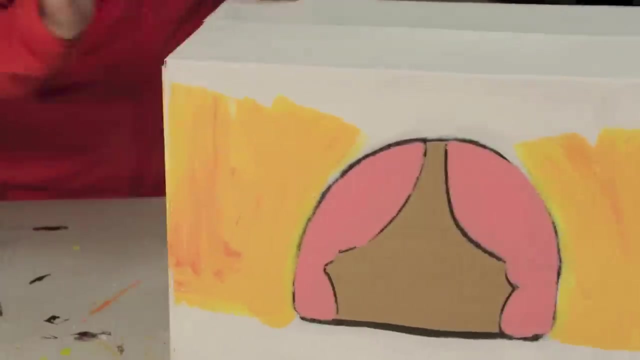 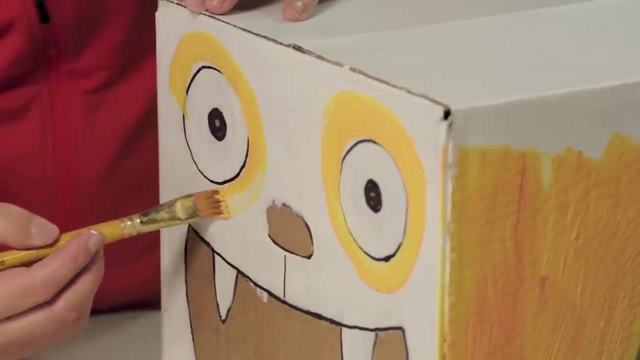 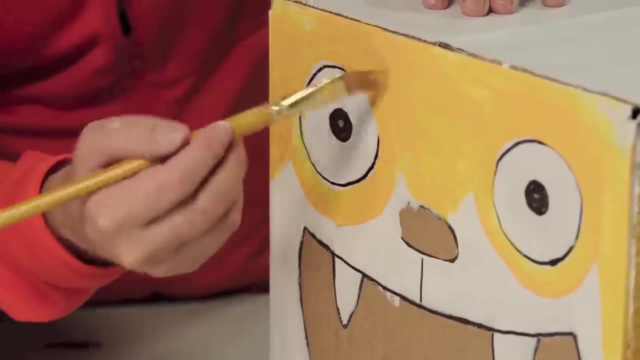 Tigers usually have a white tummy. Let's move on to the face of the tiger. Here you can see why I painted the box white first. It really makes other colours look stronger and clearer. Swap to a deeper orange and add a new layer of colour higher up on the body. 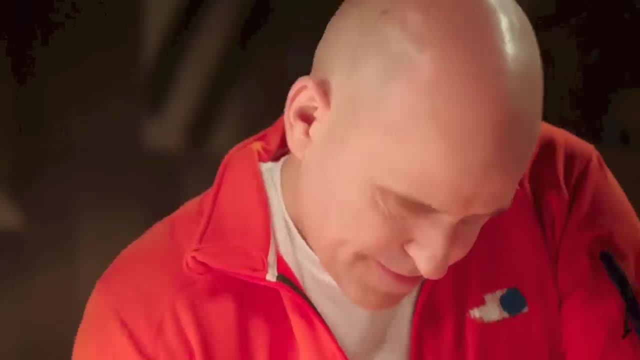 Swap to a deeper orange and add a new layer of colour higher up on the body. Swap to a deeper orange and add a new layer of colour higher up on the body. Now we have three colours: White at the bottom, A yellowy orange. 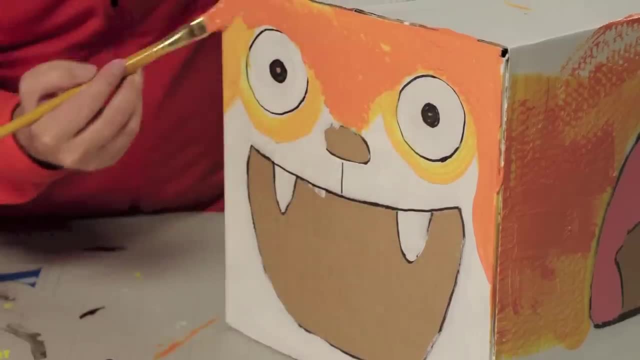 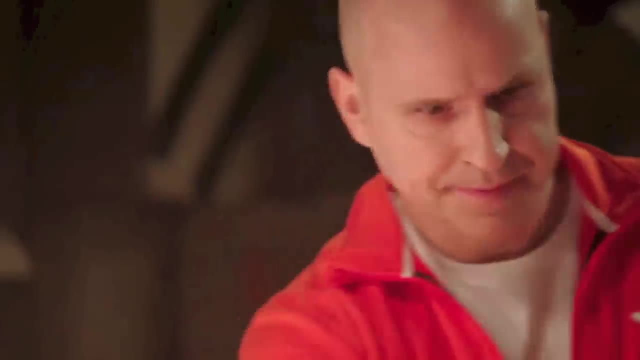 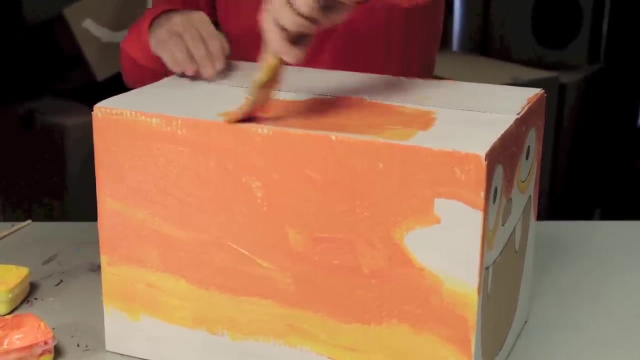 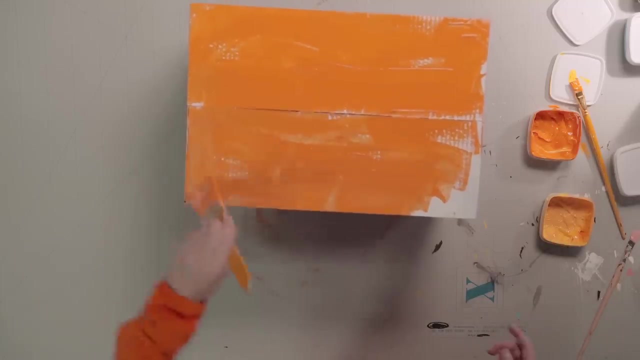 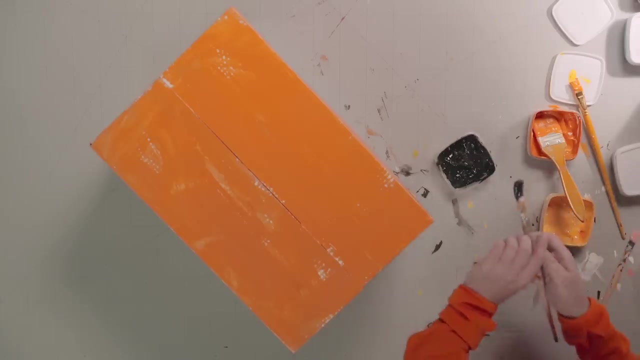 And a stronger orange And a stronger orange. Using different colours like this gives a stronger and more fun effect. Using different colours like this gives a stronger and more fun effect. When that paint has dried a bit, it's time for the tiger's black stripes. 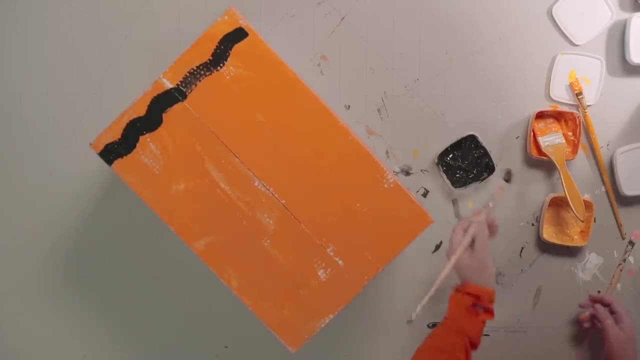 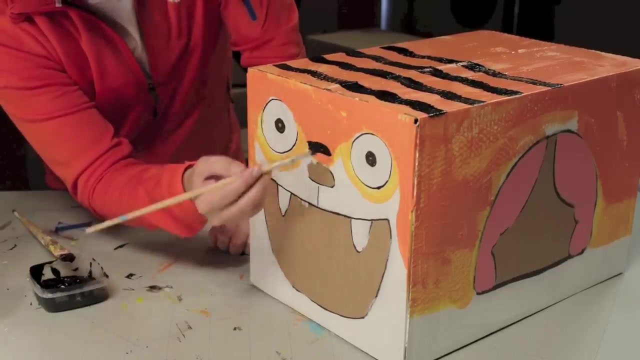 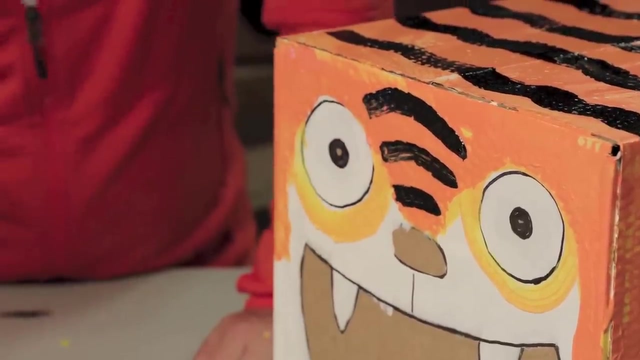 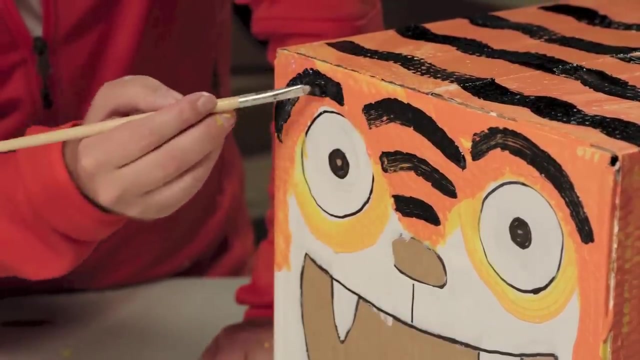 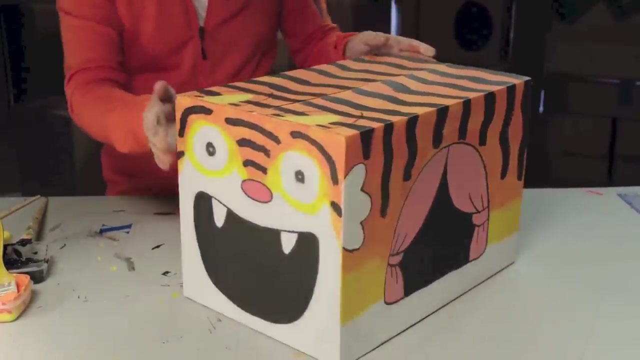 These are fun to paint because every tiger has to have cool stripes all over. I'm making them a bit uneven. it adds more life and soul. Black lines are a bit boring, aren't they? And here's a fully painted and dry tiger. 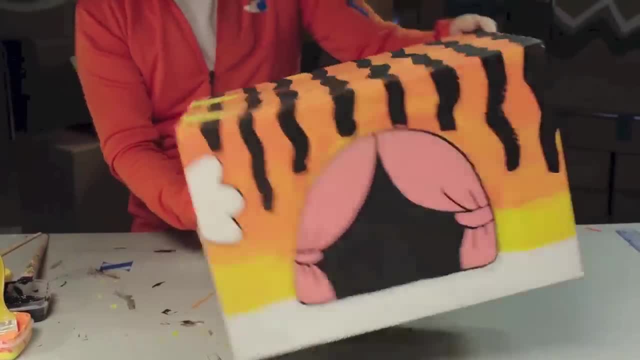 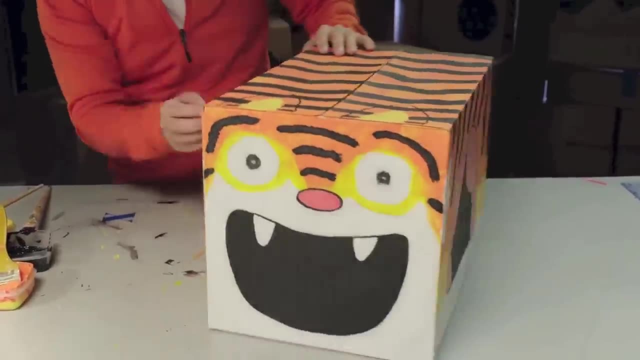 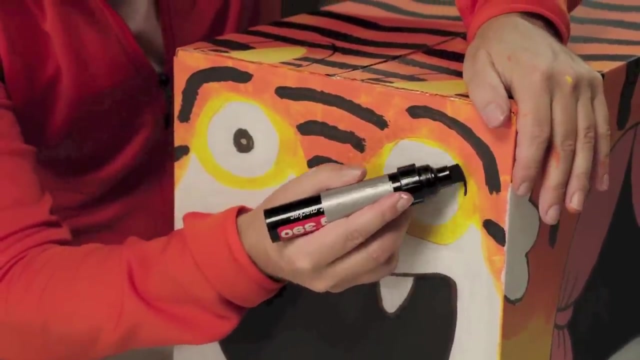 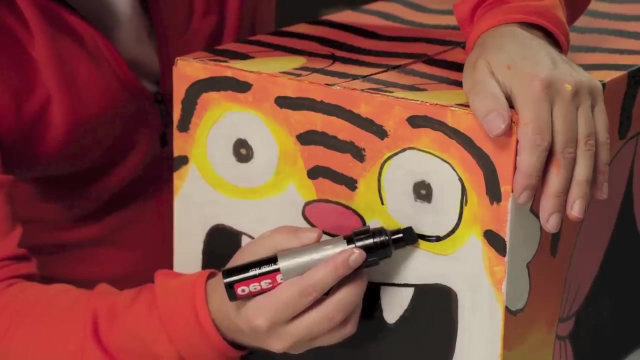 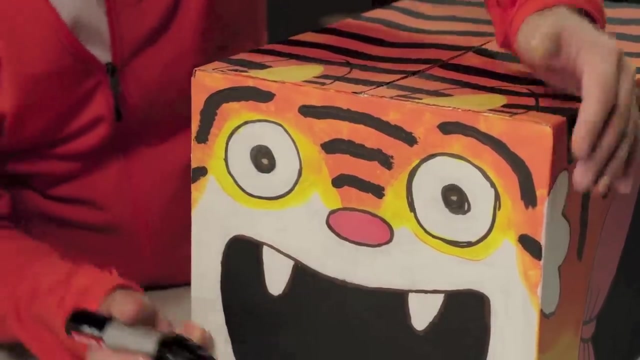 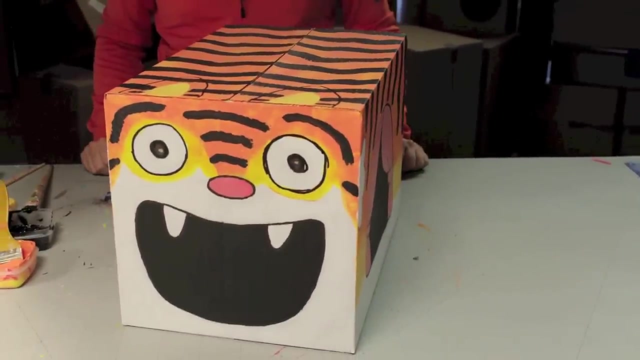 Oh, isn't it great. Oh, The last step is to get your marker pen again and freshen up any lines you've covered up with paint. This improves the contrast no end. Yeah, Your tiger is painted. Oh, Now we have a wonderful boxed cat that we can play with. 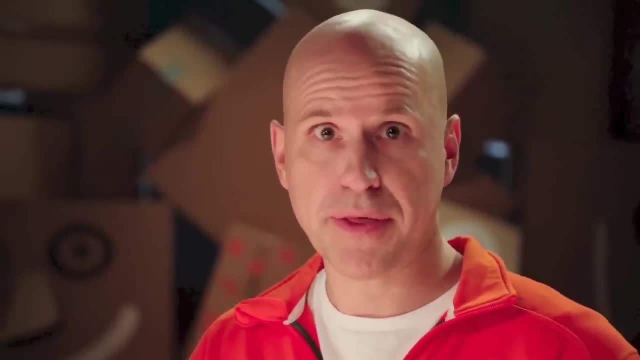 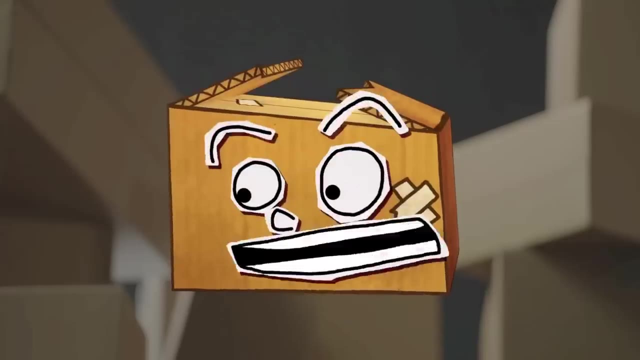 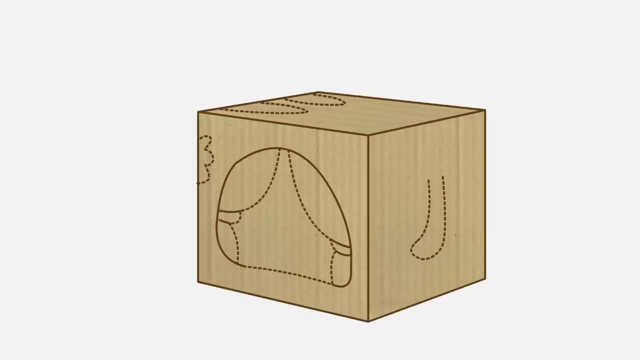 But if we want to go advanced, we continue with Cat- Then we are ready to cut the house open so that we can get in. Can you be sure to cut an extra, extra, extra large hole? Get some help from a grown up for this bit. 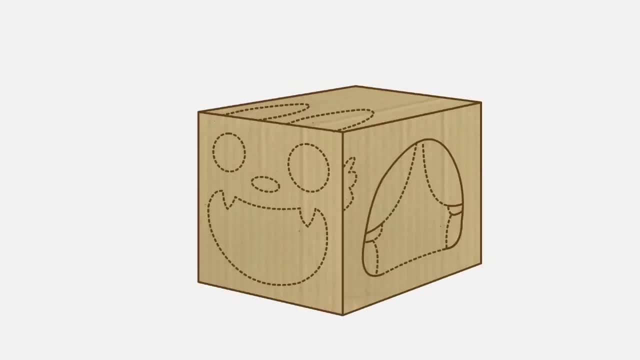 Start by cutting carefully around the tail. Then cut out the mouth and remove the cardboard. Next cut around the ears and fold them upwards. Cut out the window and remove the cardboard. Finally, fold out the tail. As you fold out the parts, the tiger really starts coming to life. 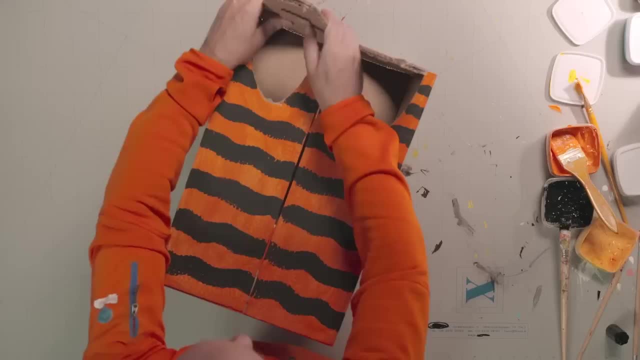 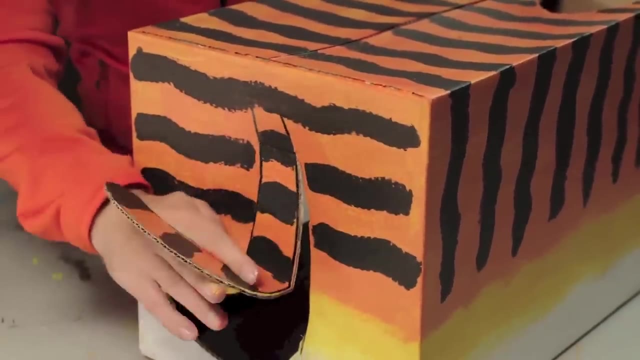 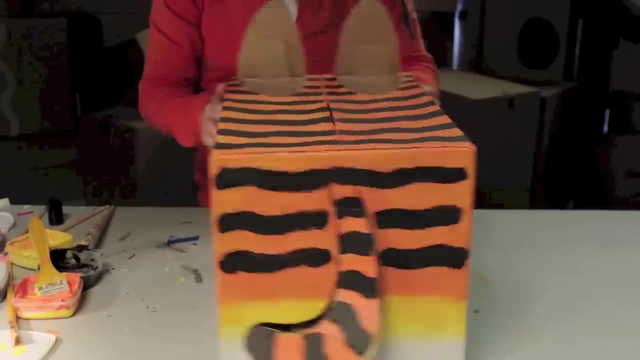 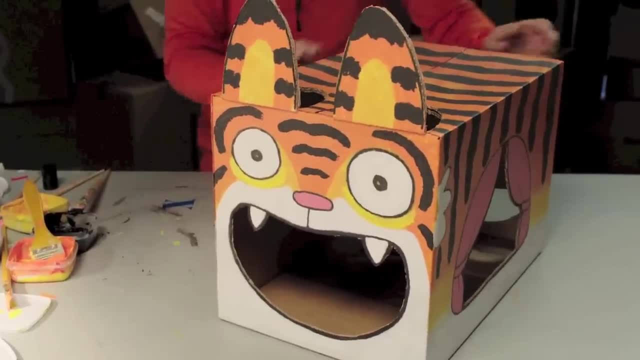 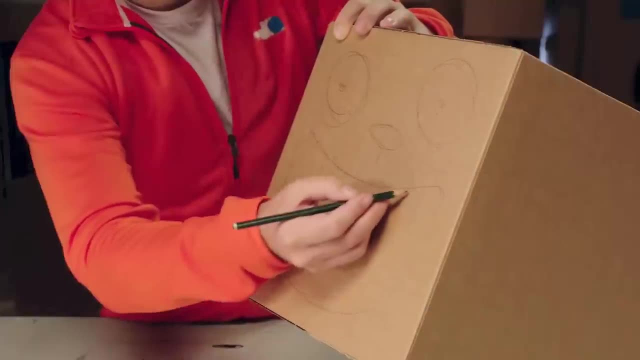 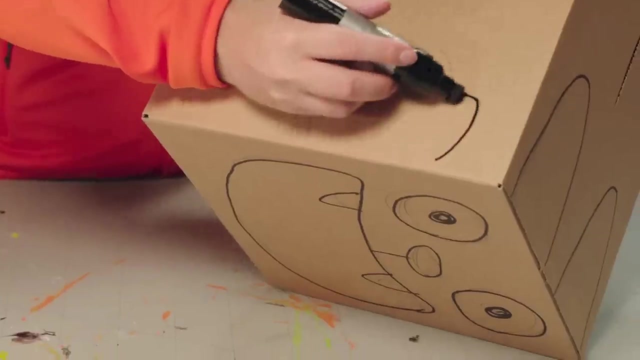 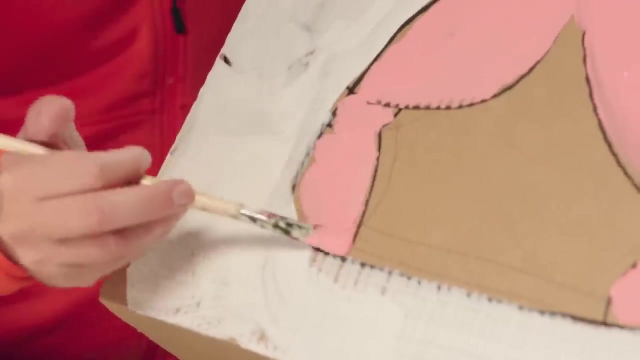 move in. All right, we'll see it one more time. Draw the tiger on the box one bit at a time, First with a pencil, then with a marker pen, Next, Next paint: a white primer layer, then pink curtains and then two layers of orange paint. 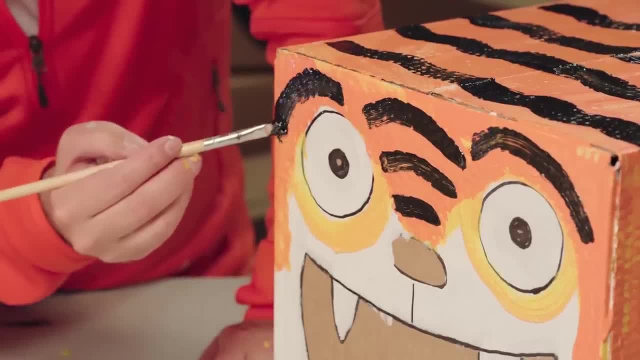 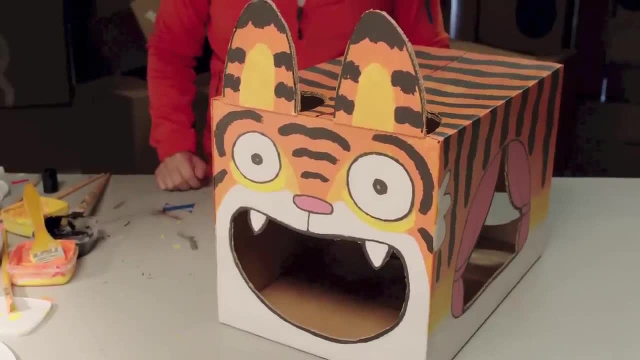 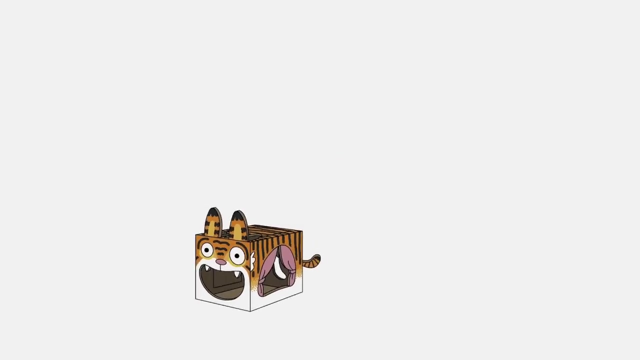 Finish up with black tiger stripes. Finally, cut fold and open up the house ready for your cat to move in. You can also turn the cat house into a cat castle. First remove the top of the tiger house, Then extend the house with several other large boxes. 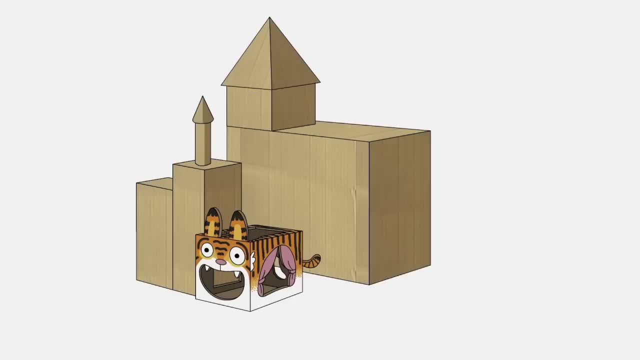 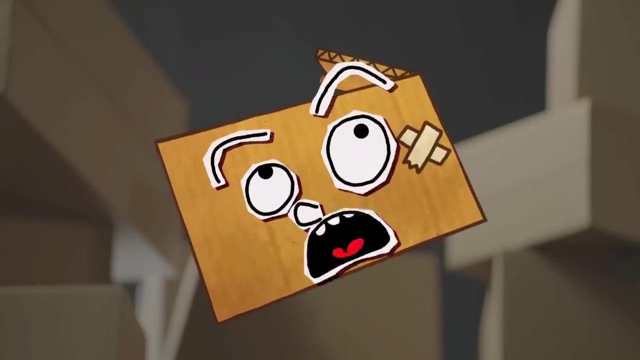 Make ceilings, doors, windows and bridges. Paint the whole thing in bright colours and your cat will live like a princess OK Box. do you have any more ideas for us? Sure thing, You can use the same method to make other pet houses, such as this mouse maze with lots of rooms and doors. 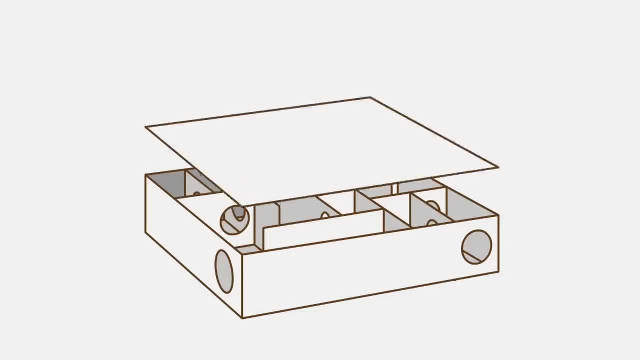 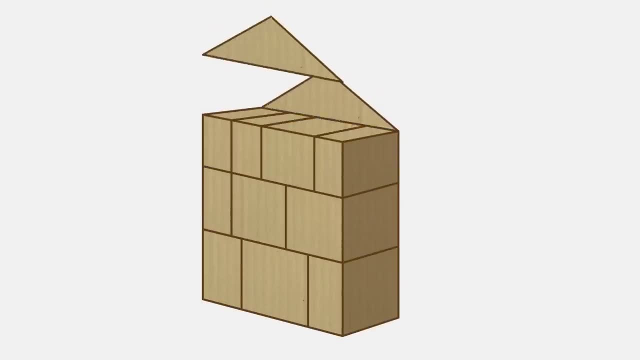 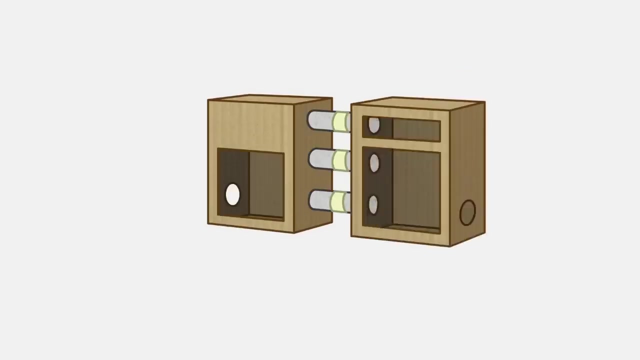 Or how about this, A birdy hotel made from loads of boxes, with a roof on top and pencils for the birds to stand on? Or this rat run put together with a couple of boxes, plastic windows and as many toilet rolls as you can find? 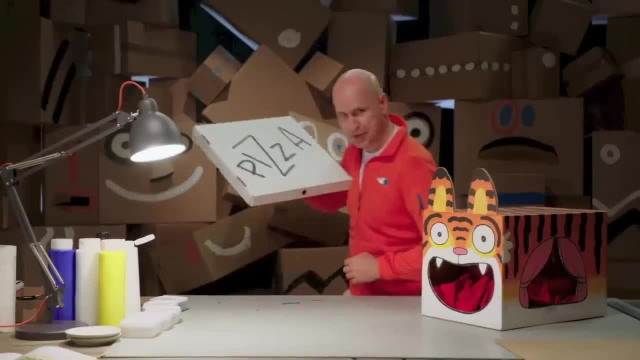 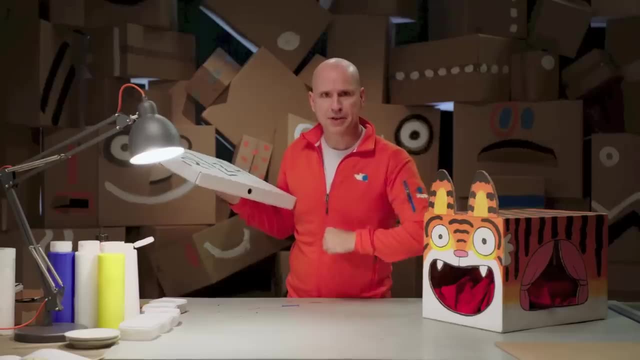 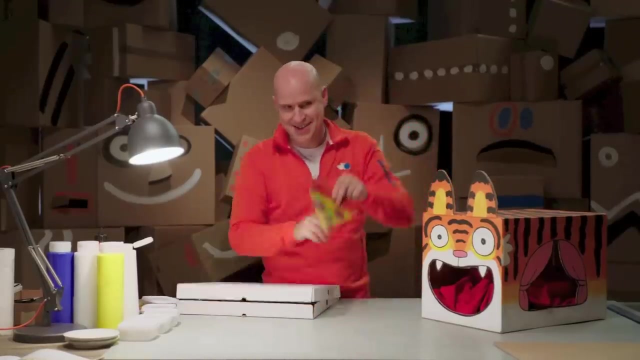 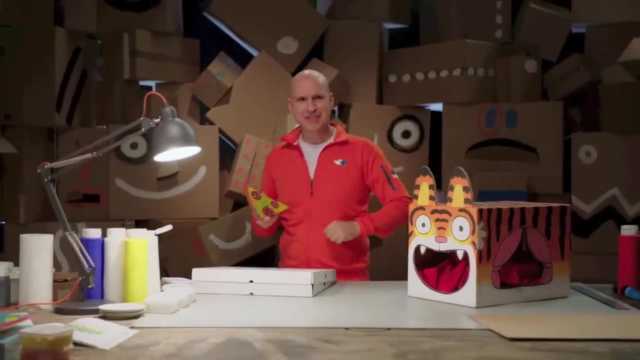 Sorted Easy Pizza delivery. Hello, anybody home? Hello pizza- Well, looks like nobody there. Better eat it myself, then. Cheers, There are thousands of ways you can box yourself. Just use your imagination And they all can be done. 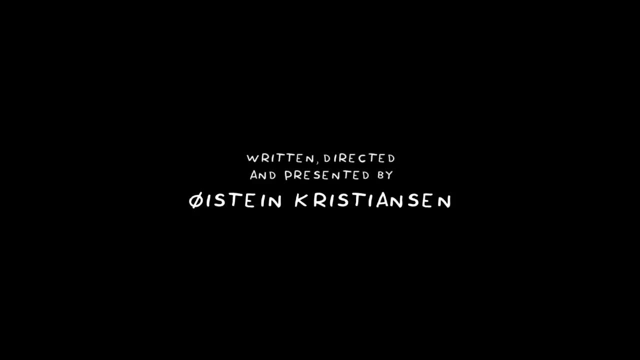 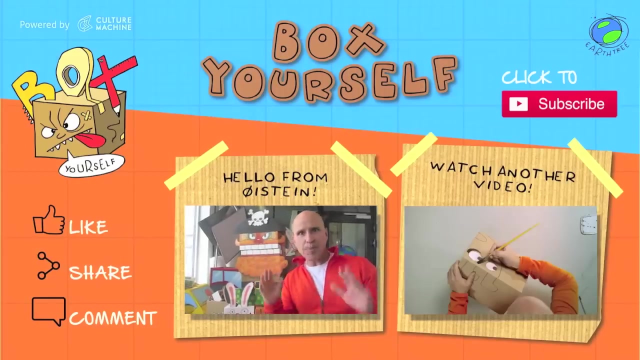 Sorted, Ah, Hahaha. Hello, I'm putting up new videos here all the time, So come back and check out the new stuff.